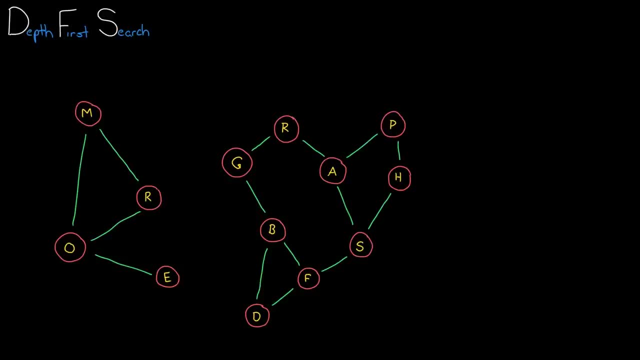 Now you basically are asking the question: hey S, do you have a path, Do you have a path to node T? And S says, hmm, I'm not sure, Let me go ask my children. And first S goes to node A and it says: hey A, do you have a path to node T? If you do, then hey, I'm done. 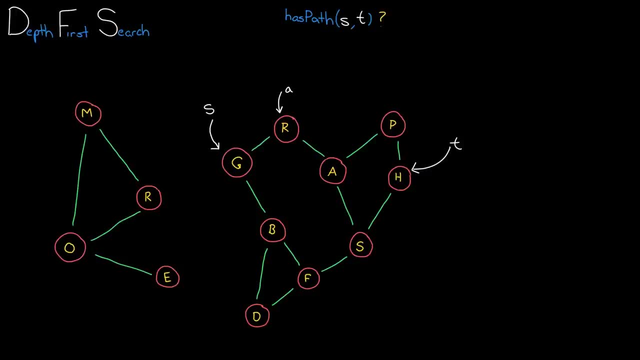 I can give you my answer. If you don't, then let me go ask B, and then C, and then D And so. but the very first person we ask is A, So A gets asked. hey, A, do you have a path to T? 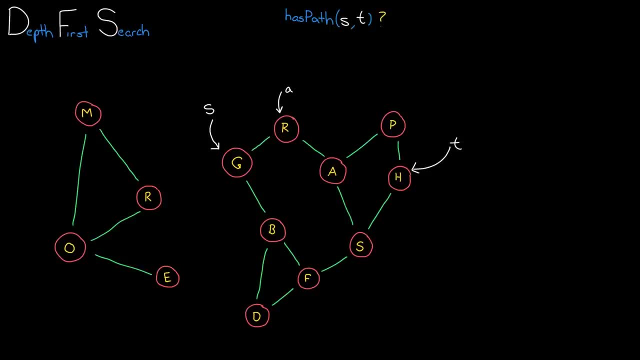 I'm not sure. Let me go ask my children, And eventually we might get to a node. who says why? yes, of course I have a path, I am T, And so then we go and say boop boop, boop, boop. 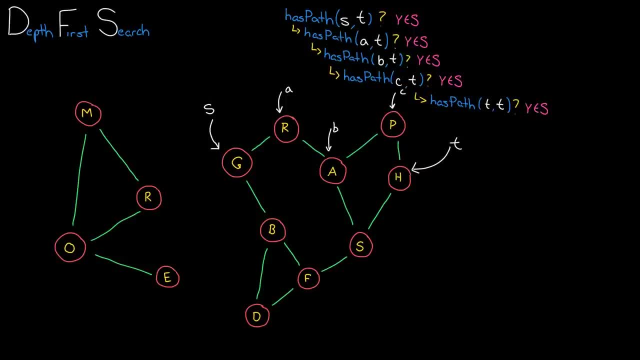 all the way back up. yes, there's a path, And that's the basics of depth-first search. It's called depth-first search because we go deep into some node before we even ask any of the children. Now, the problem with this is that we don't have a path to T. We don't have a path to A. 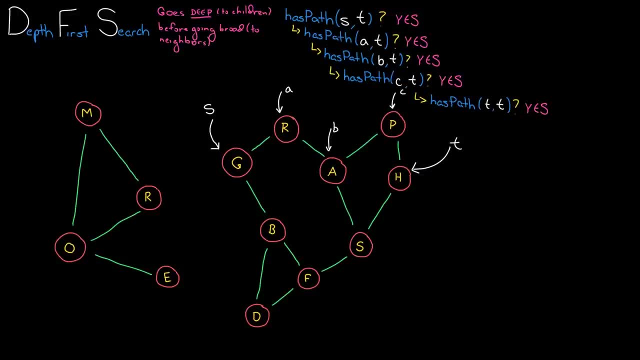 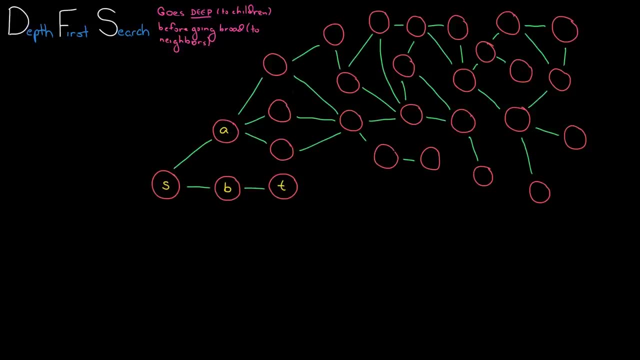 We might run really really far away. So imagine, for example, that B actually has a path directly to node T, has an edge directly to node T. A might go to all of its children, all of its children, all of its children, before you even get to B, and T was right there. There could have been a. really 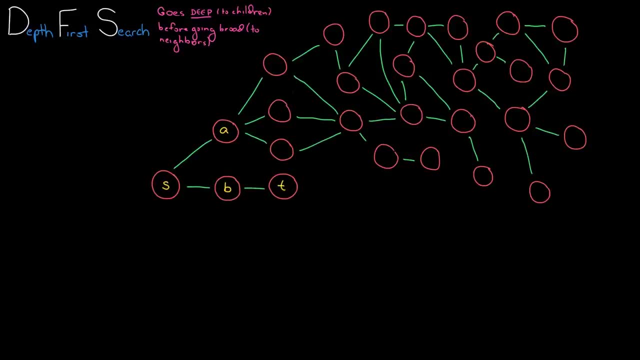 fast connection. So that's why we might often prefer to use breadth-first search instead. Breadth-first search says, hey, go level by level out. So first we ask S, hey, do you have a path to T? And S will say, well, let me check if any of my 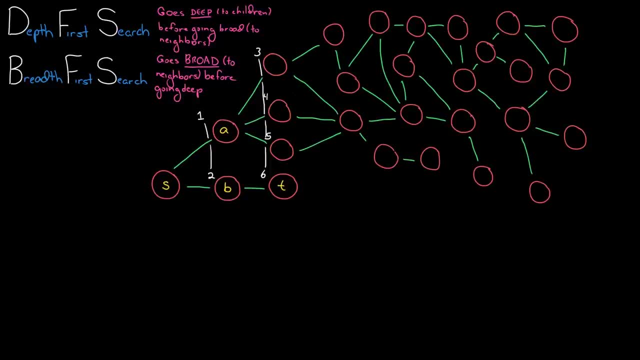 nodes are T. No, there's no edge right there, So each of those get in line, And then we ask the second level out, and then the third level out, and the next level, and next level, and the next level, And so we go level by level breadth. we go wider before we go deep, And that's why it's 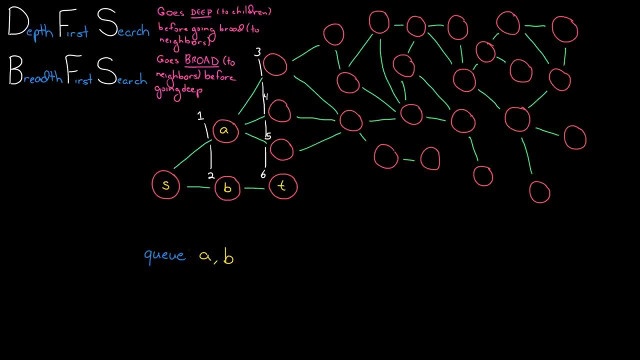 called breadth-first search. So I want to talk at a high level about the implementation of each node and then I want to dive into some of the details. So breadth-first search is implemented with a recursive algorithm. It's probably the simpler algorithm to implement, The only little. 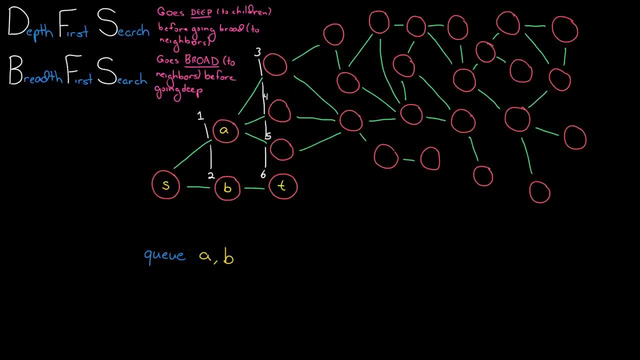 trick is that you have to make sure to use an is-visited flag so that you don't wind up in some sort of infinite loop where there is a cycle and you keep asking each node if it has and you start running around in a circle With breadth-first search. the main trick you need to remember is: 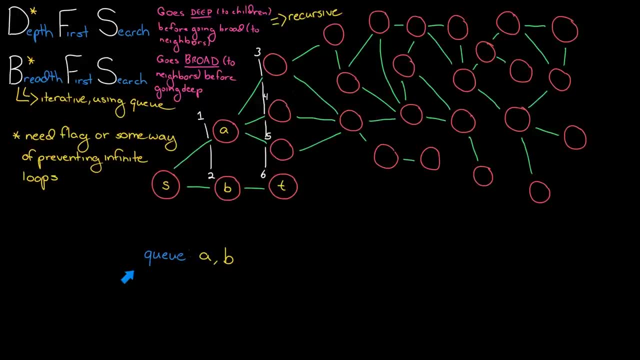 you want to use a queue. So when you use a queue, you want to use a queue. So when you use a queue, when you look at s and you say, hey, do you have a path to t, you're going to go add all of its. 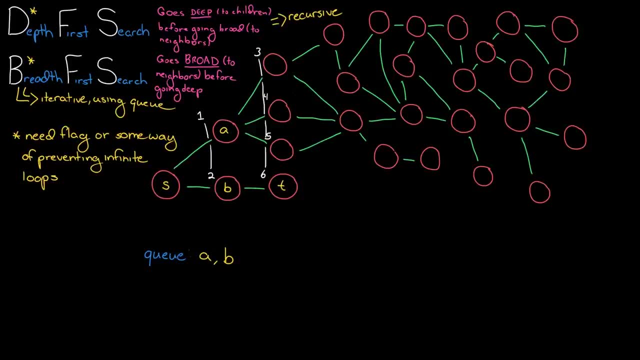 children to the queue And, rather than going recursively, you pull out the first element from the queue, check if it has a path, check if it is this final element and if not, go add all of its children to it. So you use a queue so that you go through things in the correct order. 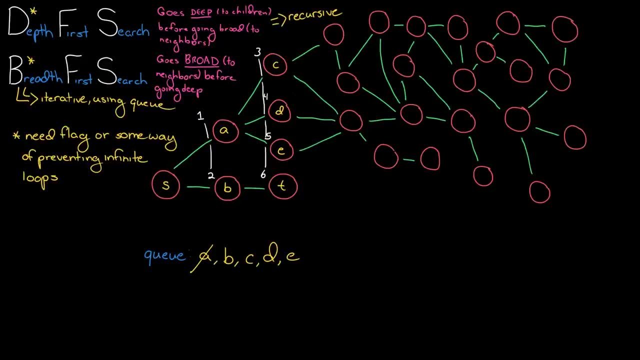 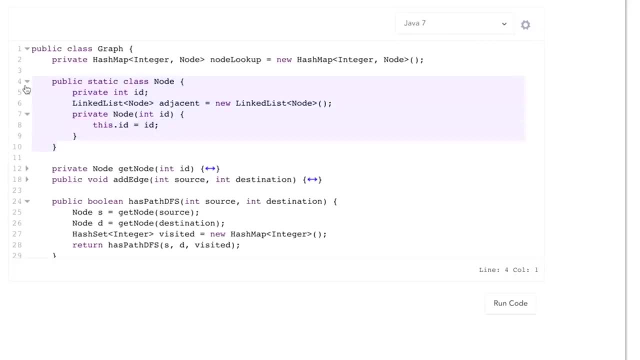 So that's the high level, how it works. Let's turn to the real details of the implementation. now I've gotten a bit of a head start on the implementation, but I'll show you just quickly what I've done. So first we have this node class here and it's going to have some sort of ID that 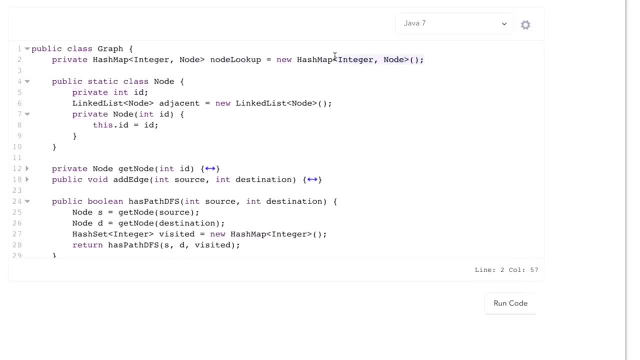 represents the node ID, And what I've done is give ourselves a mapping of from node ID to the actual node, And this is mostly going to be used for things like get node and add edge. This way we can actually just go and get immediate access to the node with a particular ID. And then I've also given 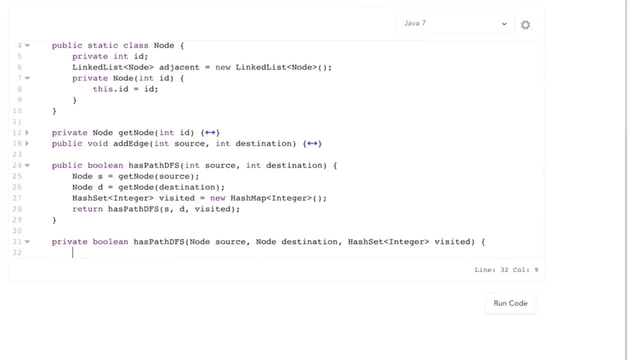 us. this has path depth first search method and it's going to call after this recursive method. So if you remember, with depth first search we need to have a way of flagging nodes to say, hey, I've already visited this, don't retry it. So one thing we could do is we could actually 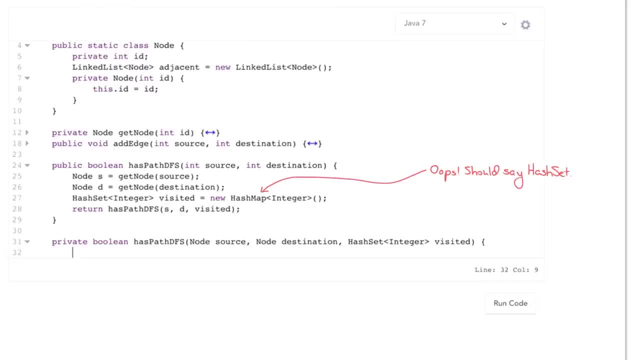 modify the node class to give ourselves an is visited flag. But that requires then making sure we clear that flag later on. Another way of doing it is giving ourselves a hash set that lists the IDs that I've already of the nodes that I've already visited. It's sort of a replacement for a. 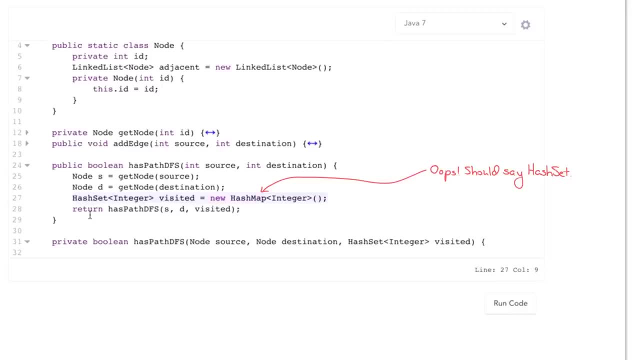 flag. So I'm going to do it this way. This way I don't have to modify and add a whole bunch of flags in and then make sure to clear them later on. So I get the source node, I get the destination node. 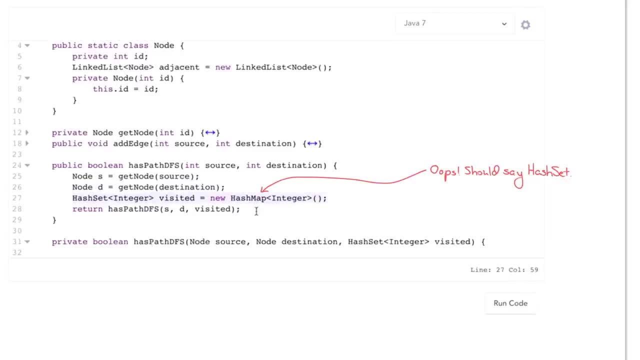 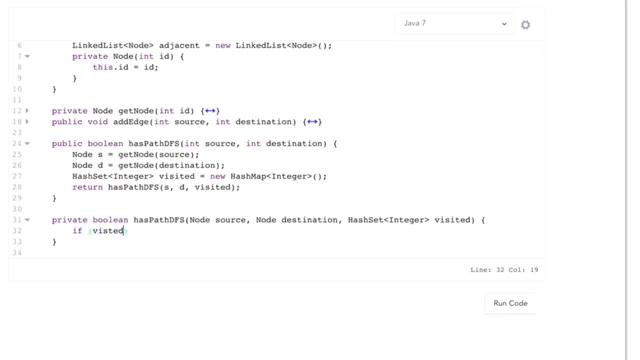 And then I get this: create this visited hash set, And then I go out and call the this recursive method. So now is where the fun begins. So first, if I've already visited this node, if visited dot contains this source ID, then return false because there is no path. then 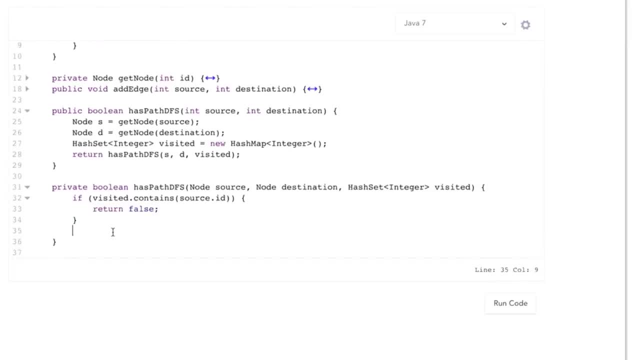 Okay, otherwise then what I want to do is: so now I want to go and make sure I, you know, update this mark, this node is visited, And then I want to say, okay, if, if I'm at my source, then return. if I'm at my source, then I'm going to say, okay, if I'm at my source. 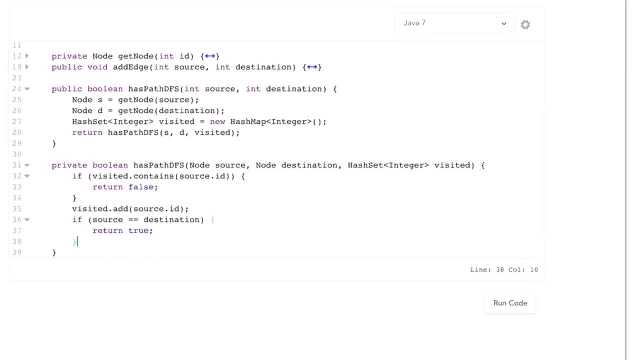 I'm at my destination rather than return. true, because, yes, there's certainly just a path. then, Otherwise, go and check all my children, see if any of them have a path, because if there's a path from a child to me, then then there's certainly a final. then there's certainly a path from me to 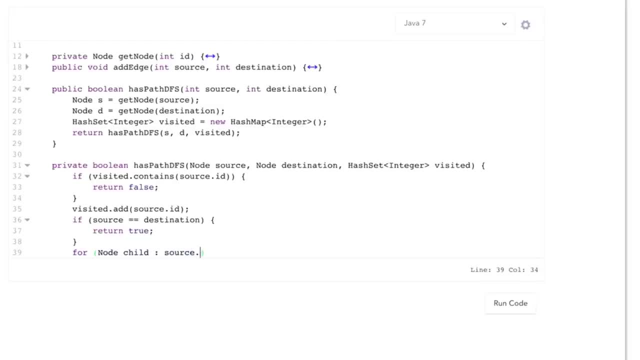 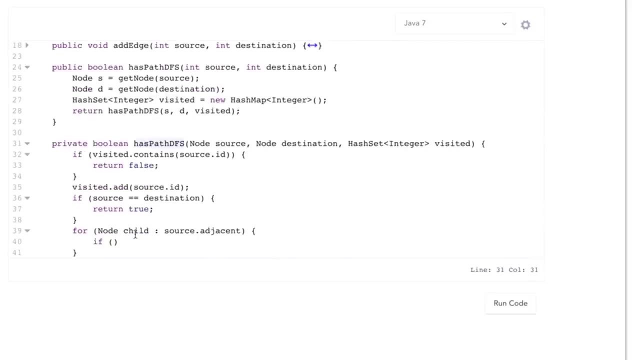 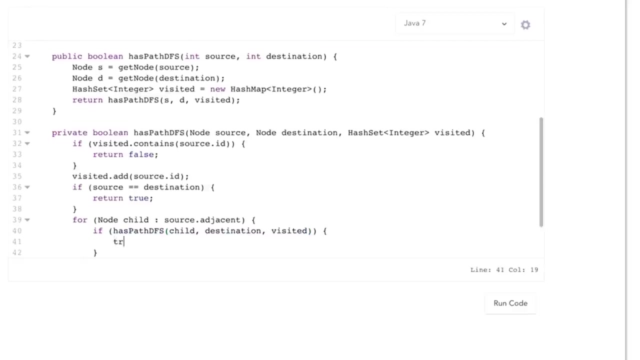 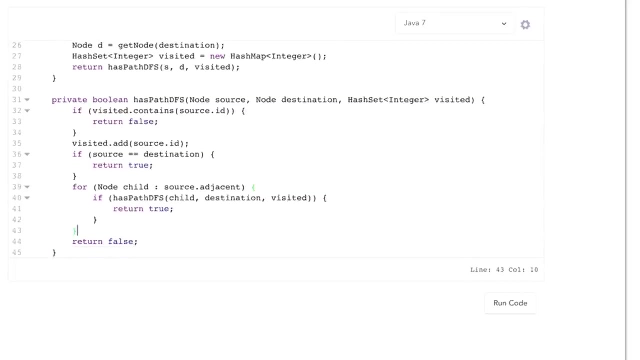 my destination, So for each node child in source dot adjacent, if there's a path from child to destination passing in, again visited, then return true, and that'll bubble all the way up the stack. If I get down to the very end and I haven't found a path yet, then there is no path for me to. 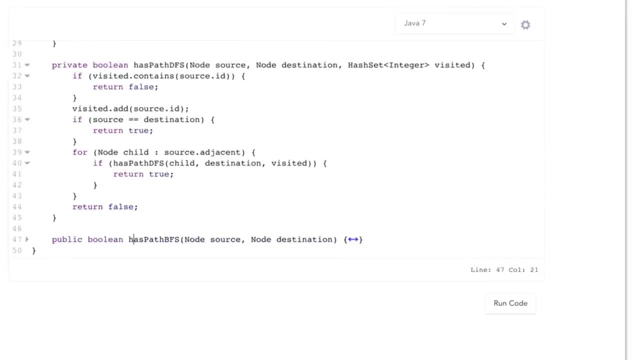 my destination. Now let's turn to how breadth first search works. Okay, so breadth first search. So what I need with breadth first search is I need a link list of sort of what I'll call the like next up. So these are the I'll call this next to visit. These are the nodes that I need to visit next. 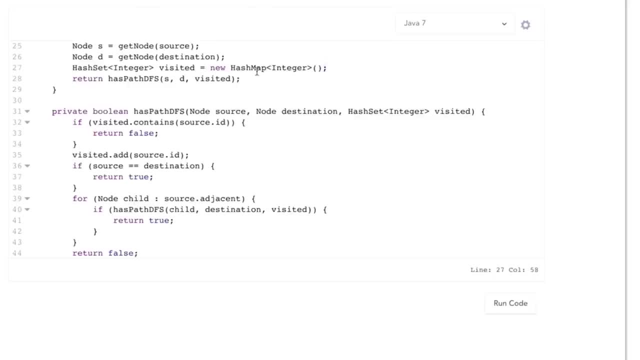 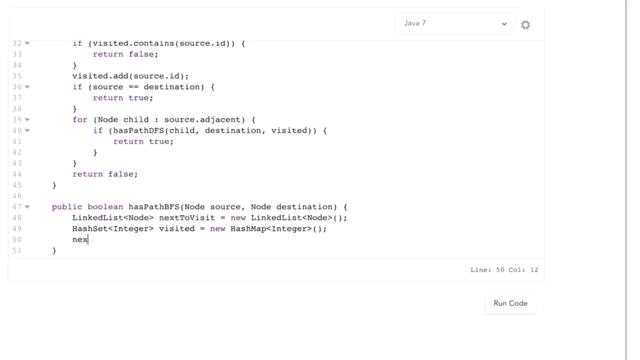 And, just as before, I need this visited hash set that represents everything I've already visited. And then I want to say next to visit, first thing, because the first thing I need to visit is, in fact, my source. Then, as long as there is nothing in there, I'm going to call this next to visit. 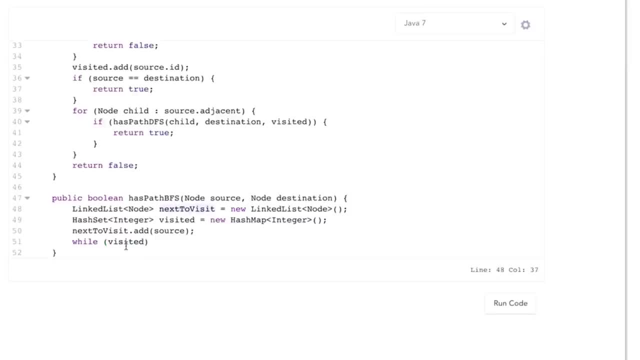 So while visited- sorry, now I'll next to visit- dot is empty. So while it's not empty, keep going, All right. so first thing, so I need to look, grab my very first node to visit. So node node equals. 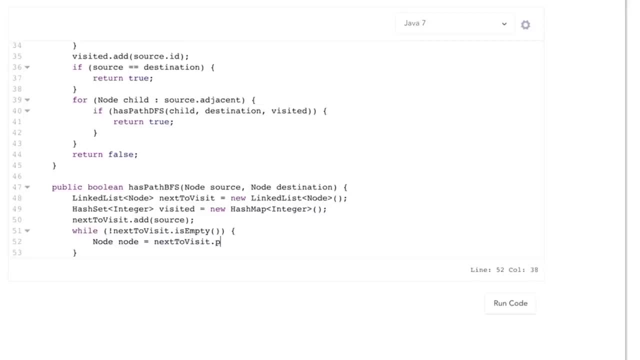 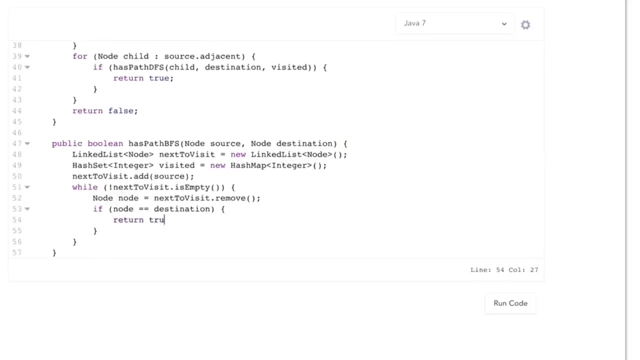 next to visit dot, I'll call this remove. So remove the very first node in that list. If this is my destination, then there is certainly a path. Now I also want to do my visited checking. So if visited dot contains of node ID, then actually just continue. 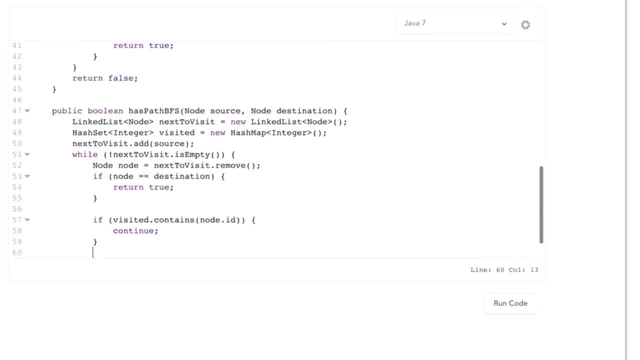 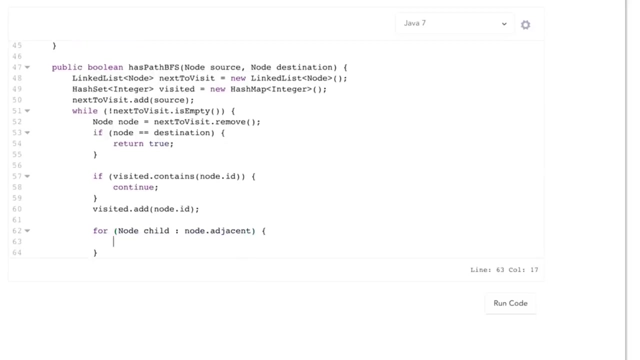 Let's go to the next value, Otherwise visited dot. add of node dot ID. So mark it as no. Okay, So mark it as visited. and then go and actually add my children. So for each node child in node dot adjacent, go and add each of those to my next to visit. 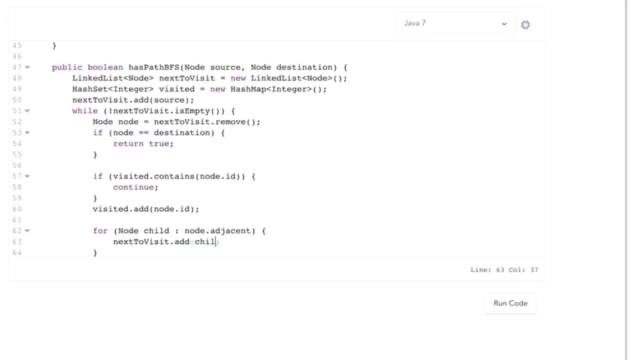 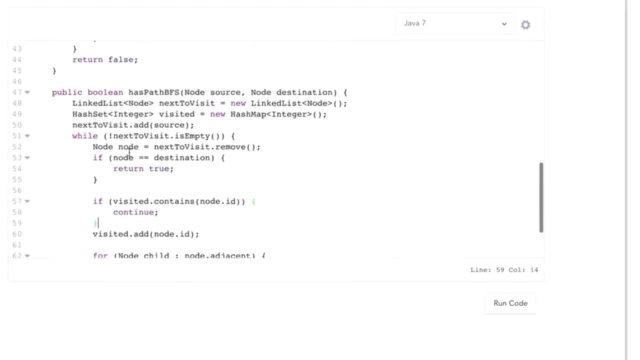 So next to visit dot: add of child. All right, and that's all there is to breadth. first search And then, of course, if I get down to the very end and I haven't found a path yet, return false. Let's walk through this code again and make sure that this makes sense. 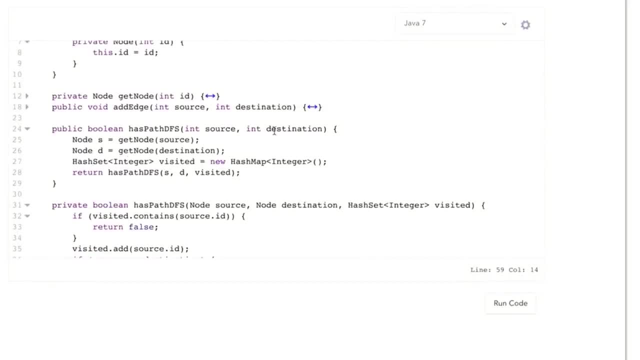 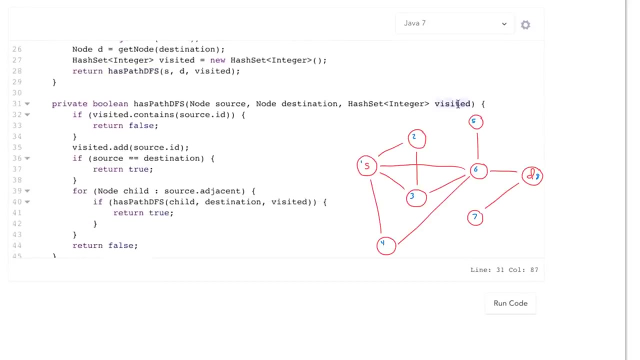 So has path DFS, takes in the source and destination IDs, and then I get those nodes and then I create this hash set- That should be a hash set, not a hash map- And then goes and actually does this recursive method. So the recursive method has this visited thing. 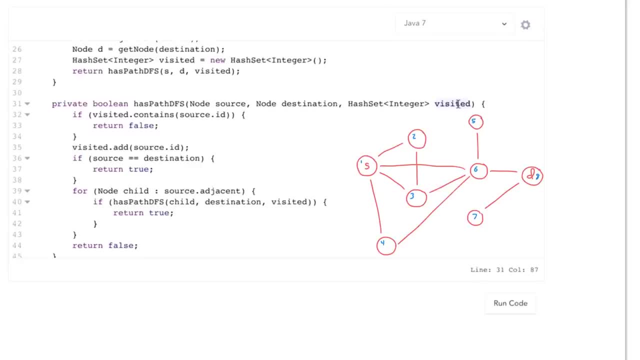 So we use the visited hash set instead of marking the actual node. So the visited check text that contains the source ID. If it does contain that, if it already visited, this return false because there's no path then otherwise go and add this visited mark. 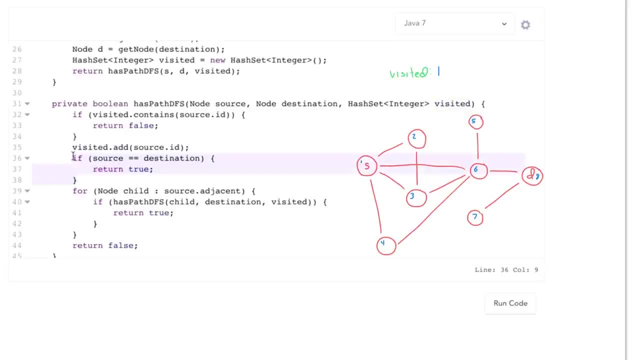 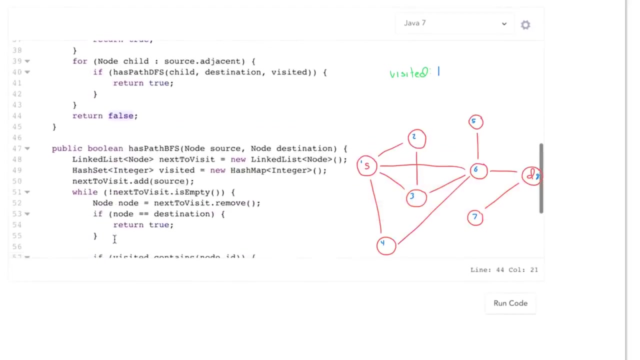 This node is visited. Check, check my sources. My destination shows me already there. Return true. Otherwise, go and search all of my children Then, so that, and then if I haven't found it, path go, return false. So with BFS we are taking in a source and a destination. So here I've used nodes. 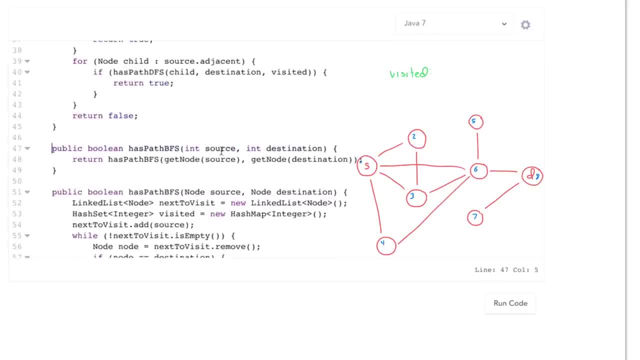 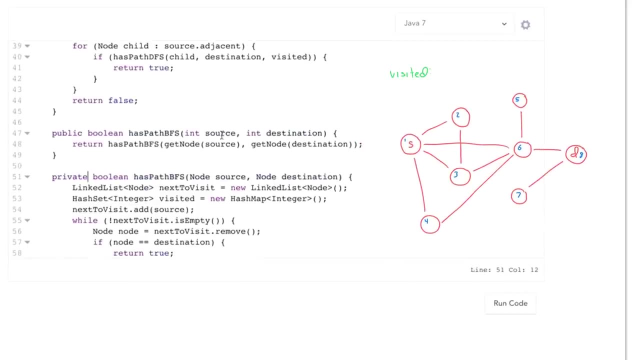 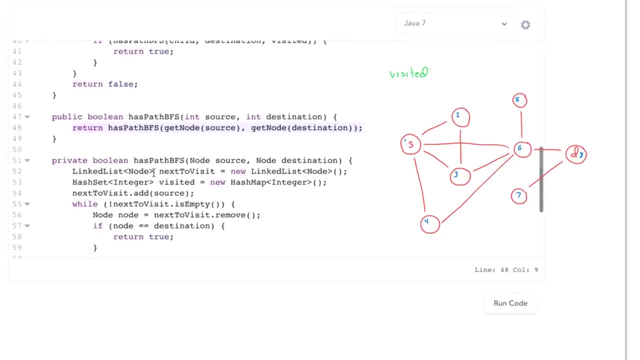 I'll switch this actually to be symmetric and use ids again, and so I'll make that public and this private. now, Okay, so I take in the source and destination ids and then I go and call this recursive method. So my recursive method, all right, sorry, this other just helper method. so this takes.